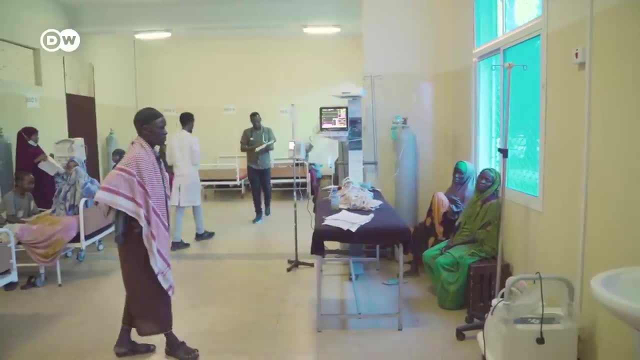 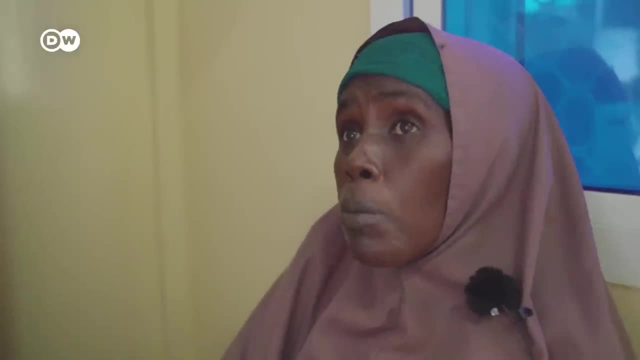 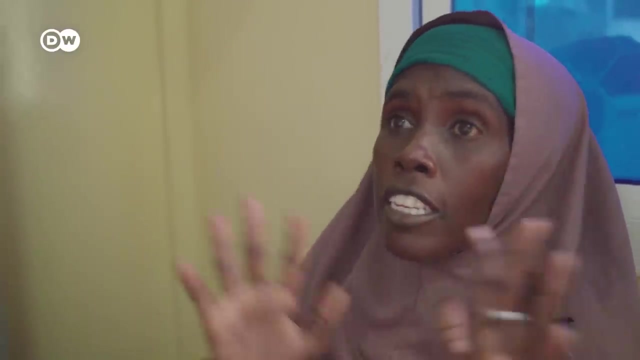 The two women have already lost three children between them. so far this year The drought has devastated their lives. We had farms and livestock, but we lost everything to the drought and lack of water. When the animals died, she says there was the beginning of the end. 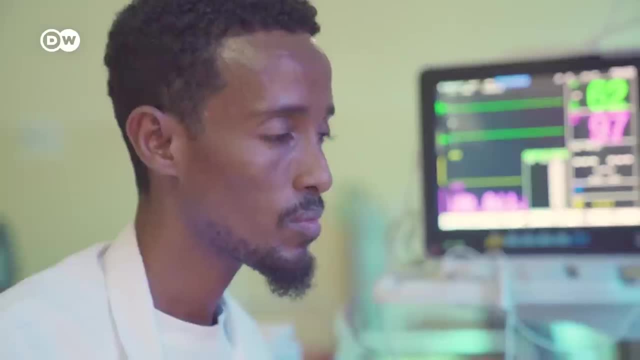 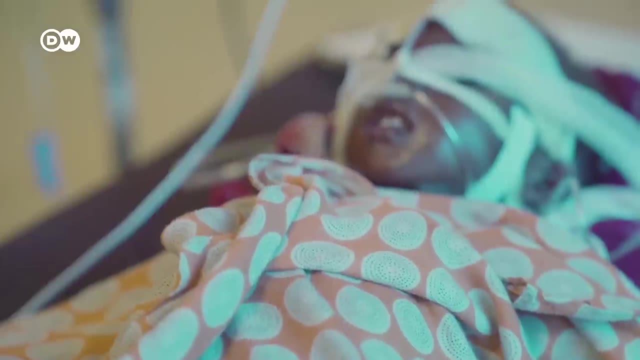 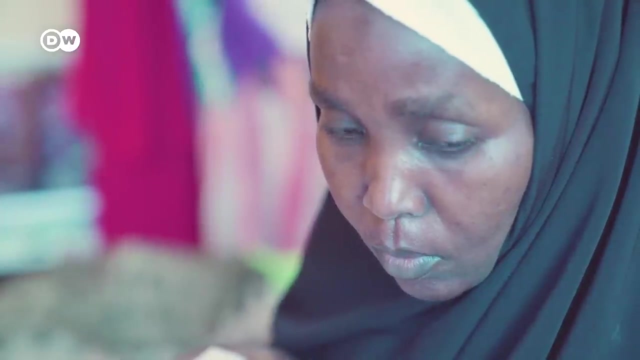 For three years we've been struggling against the drought. When it got worse, we had to come here into the city. The United Nations warns that by mid-2023, as many as half a million children under the age of five could die. 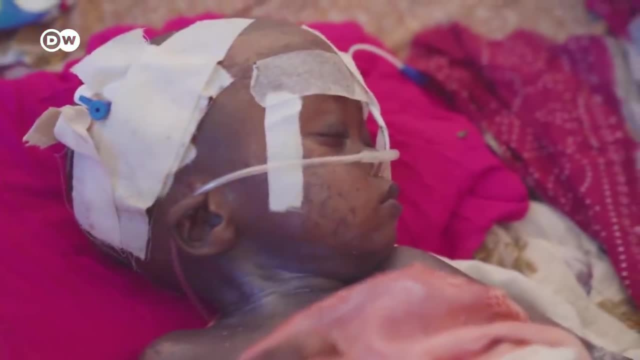 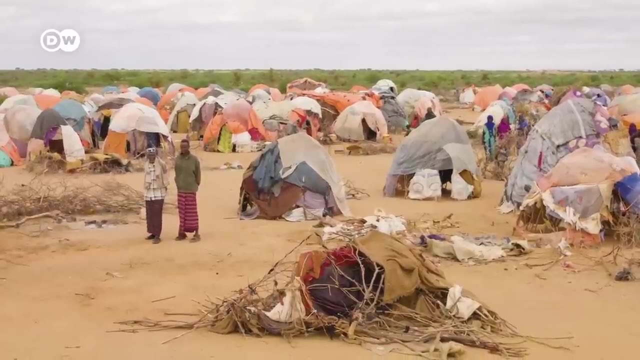 Relief organizations all agree: this is the most devastating drought in 40 years. Four rainy seasons in a row have failed to materialize, and now there's reason to fear that most of the fifth will likely follow suit. It's a disaster for Somalia's herders. 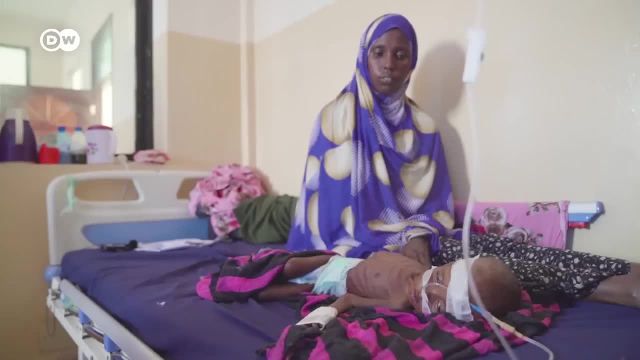 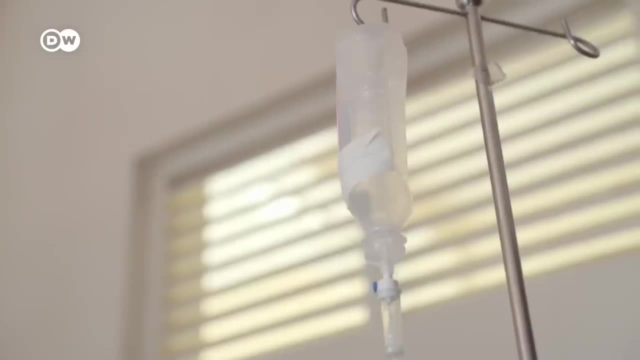 who depend on the rains. Once the undernourished mothers stop giving milk, their infants begin to starve. Malnutrition starts with vomiting, diarrhea and fevers. Often the parents don't connect the symptoms with hunger By the time they realize it. 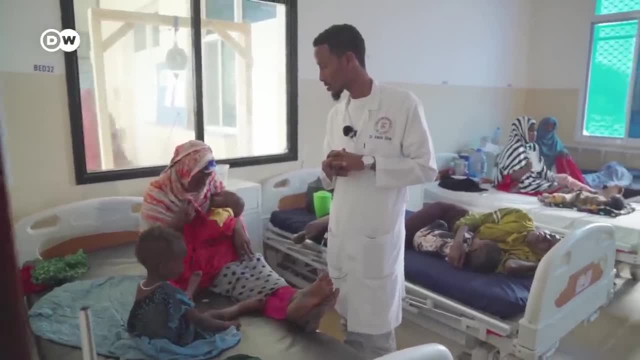 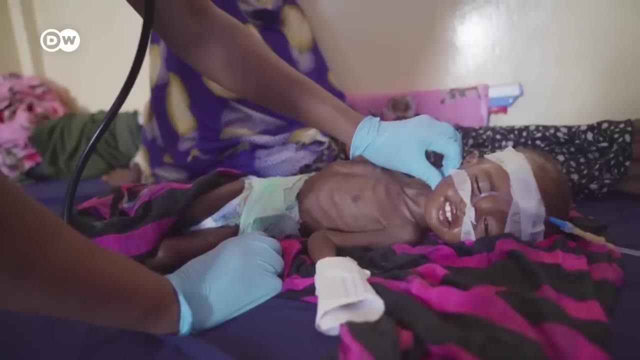 it may be too late, says Dr Hassan. Cases are coming in a terminal state, so some of them they may die. whatever you do During the first two years, good nutrition is especially critical, as this is the most important phase. 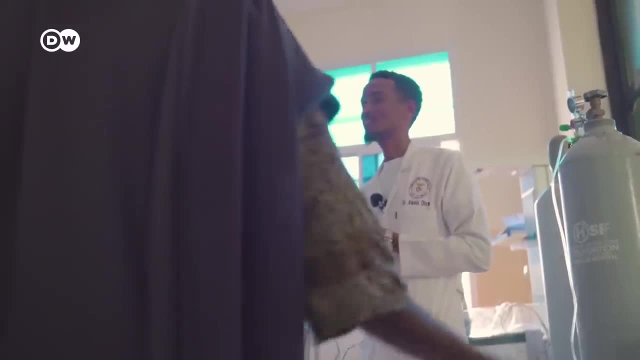 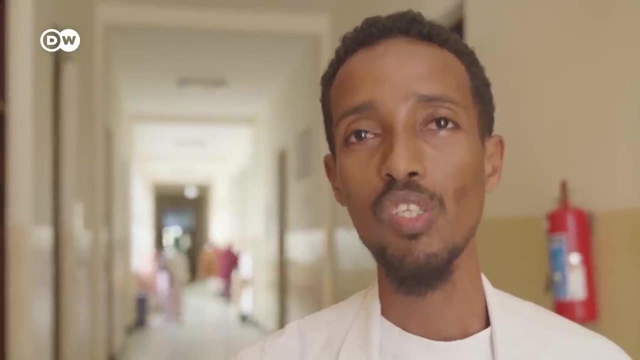 in the development of a child's brain. Dr Hassan confirms that malnourished children are highly likely to grow up with malnutrition. This malnourished child, he will not be a good president because of malnutrition, He will not be a good MB. 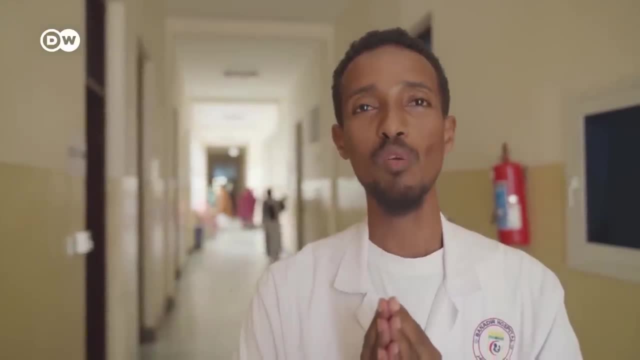 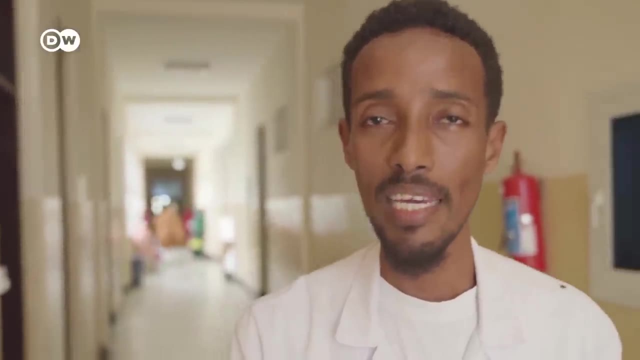 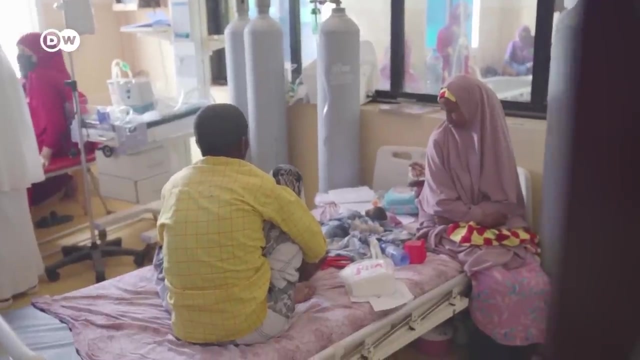 What we worry about here, not only for his productivity, economic productivity, as well as learning ability, but we are also worried about for their future leadership. We talk to Hussein, who is here with his two-month-old daughter, who is in the hospital. 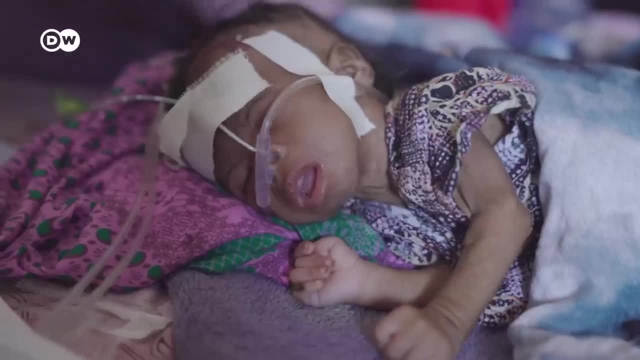 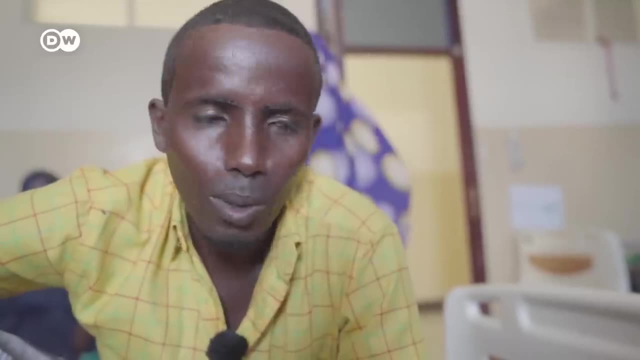 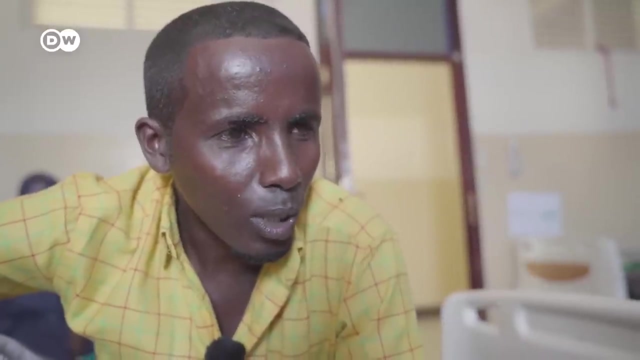 He tells us he was a farmer until the Islamist al-Shabaab militia confiscated his land. They harass people. They take your livestock and force you to join them. They say we should be fighting alongside them And anyway our livestock perished because of the drought. 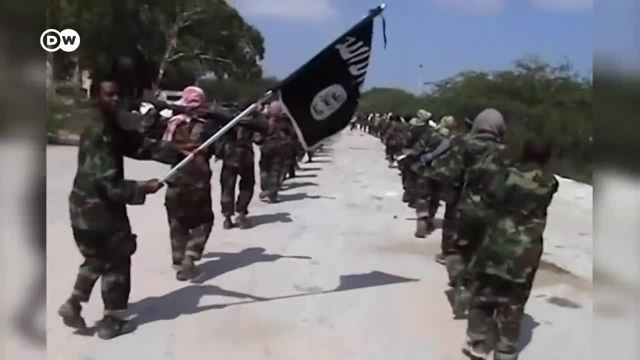 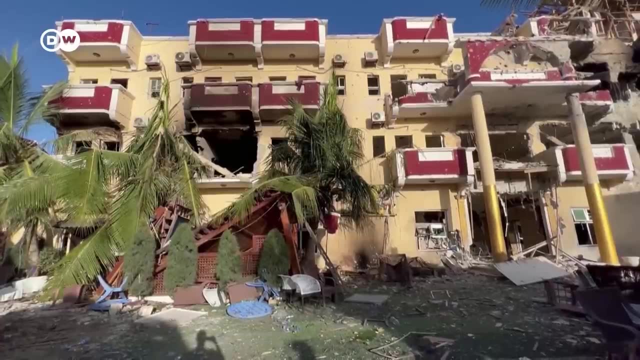 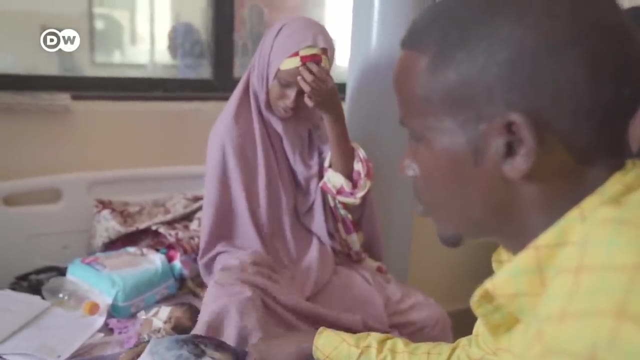 Militant Islamist group al-Shabaab controls broad swathes of Somalia and relents on the possibility of terrorizing the population with brutal attacks. Hussein says his own village in central Somalia has been under al-Shabaab control for some 13 years. 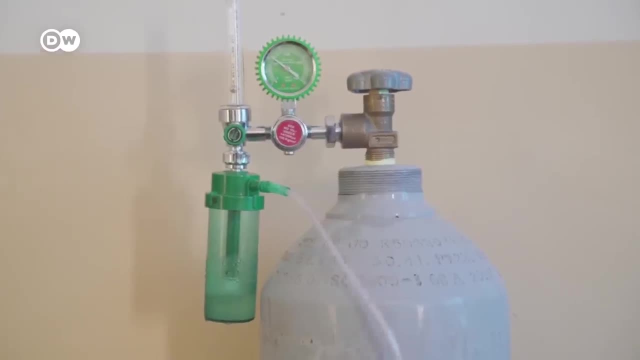 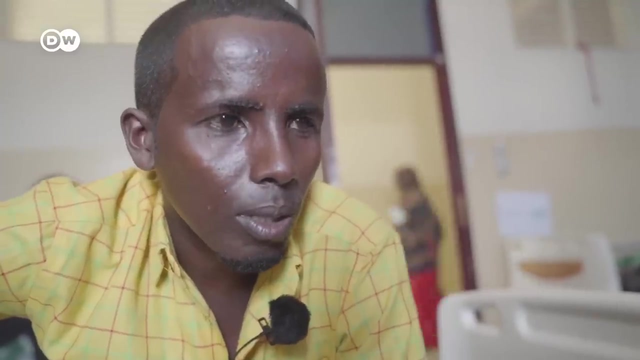 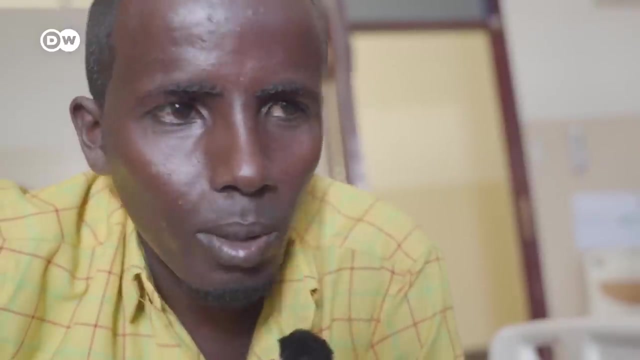 Since he fled, relatives tell him the situation has been worsening every day. People are starving and don't have enough water for their needs. There is no aid there, The government won't go there and international aid can't reach there and it wouldn't help anyone anyway. 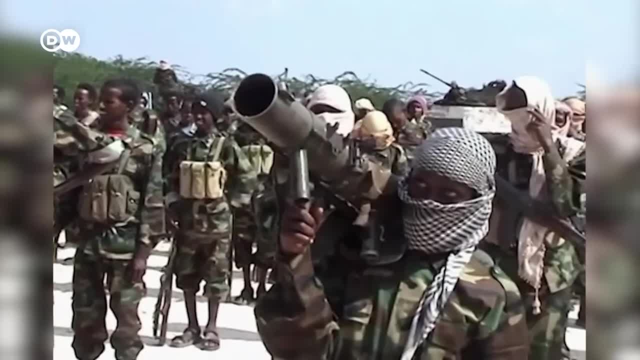 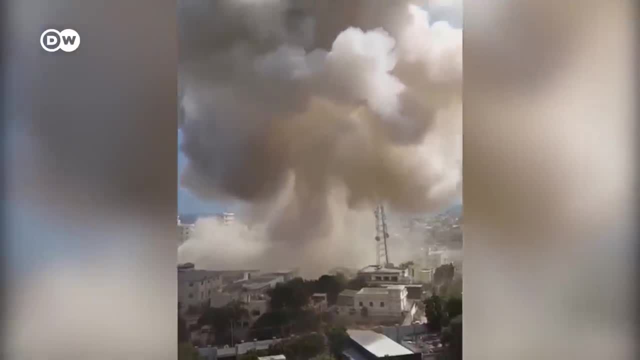 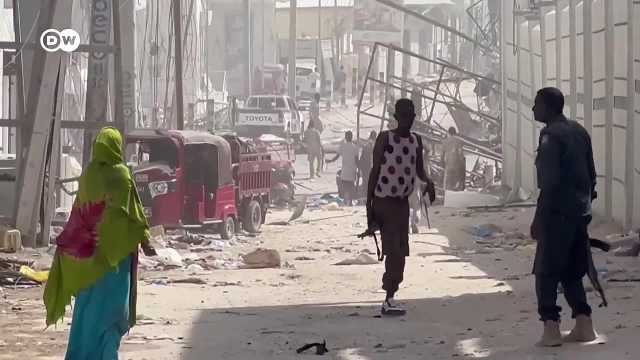 A few weeks before al-Shabaab had staged its worst attack in five years, Two car bombs detonated at a busy intersection in Mogadishu, killing over 120 people. It was the same intersection where another attack five years before took over 500 lives. 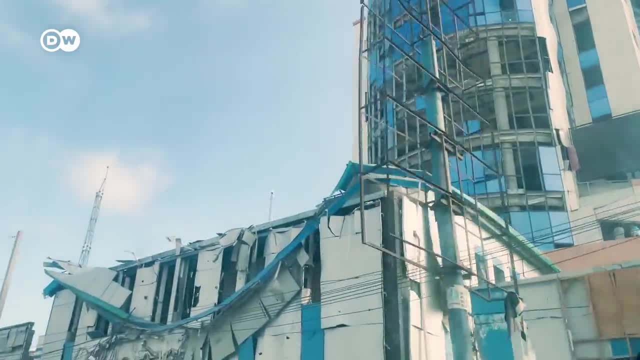 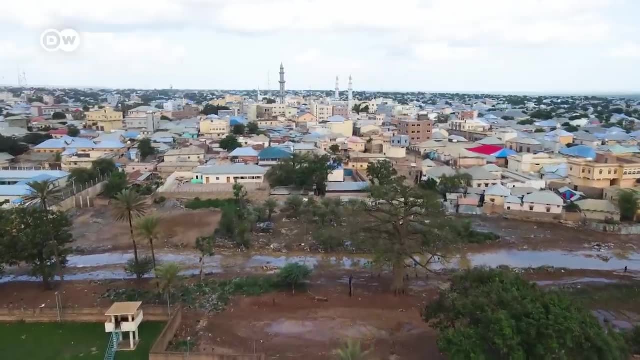 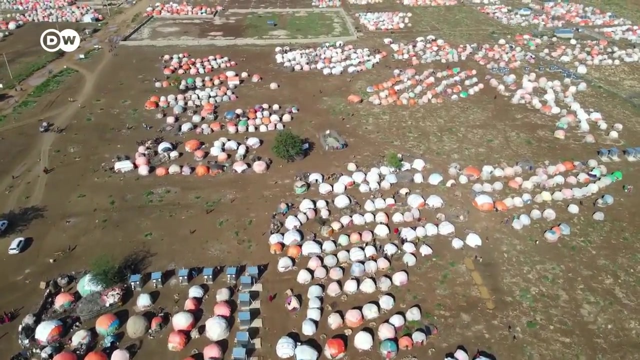 The increase in the group's violence comes in response to the government's large-scale offensive against the rebels. 240 kilometers from the capital, in Baiduwa, hundreds of thousands of people have sought refuge, Added to the city's own population of some 800,000. 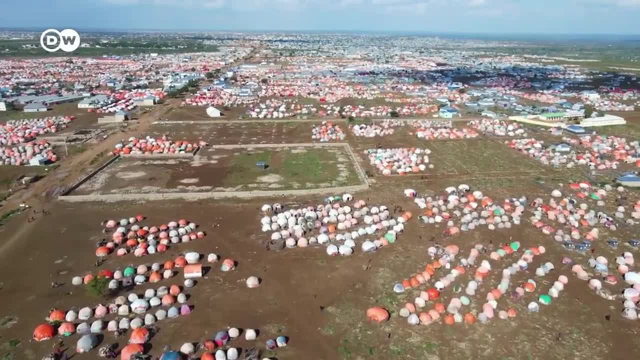 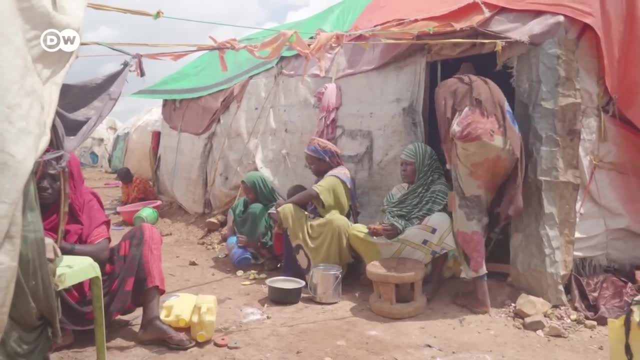 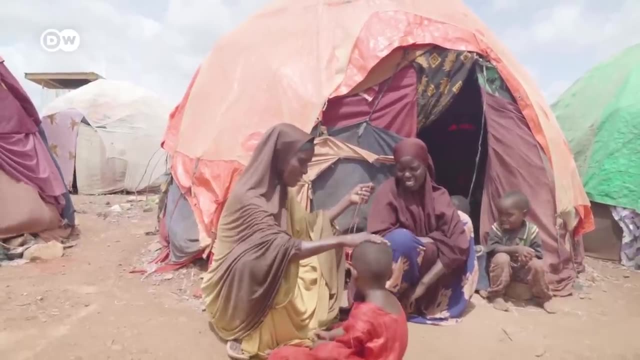 are nearly the same number of internally displaced people. According to the city administration, their numbers are expected to reach one million by year's end. One of those displaced people is Hawo Isaka. She lives in the city of Mogadishu. 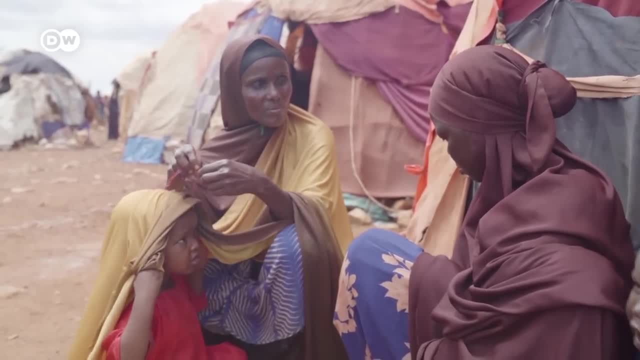 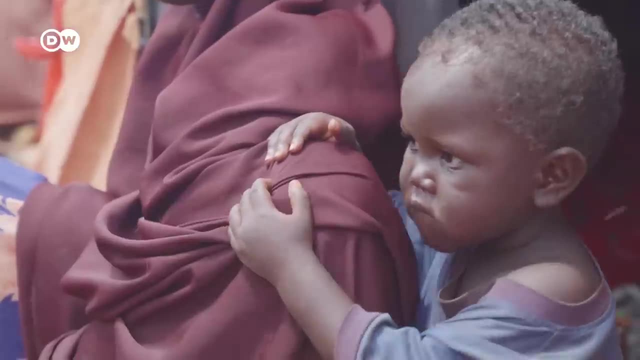 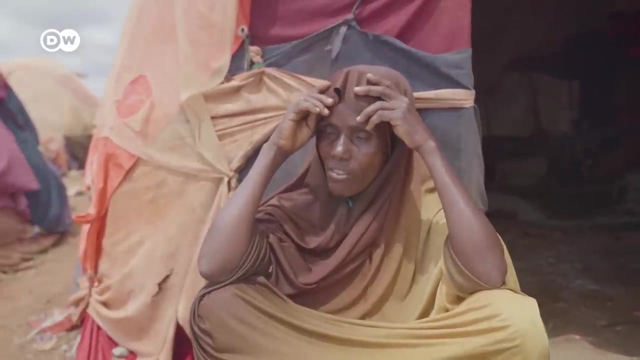 After her camels died of thirst half a year ago, she and her five children fled to the camp. We came here a long time ago because of the famine, But so far we haven't received any help. We hardly get any food or water. 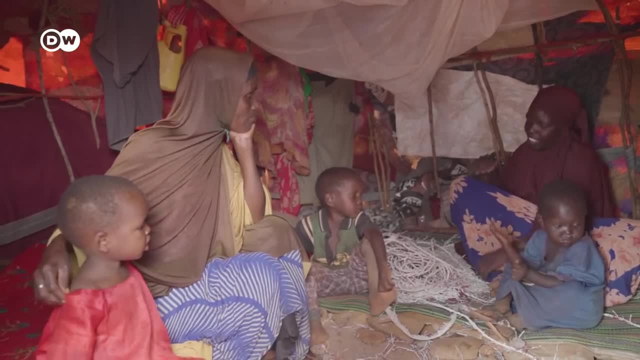 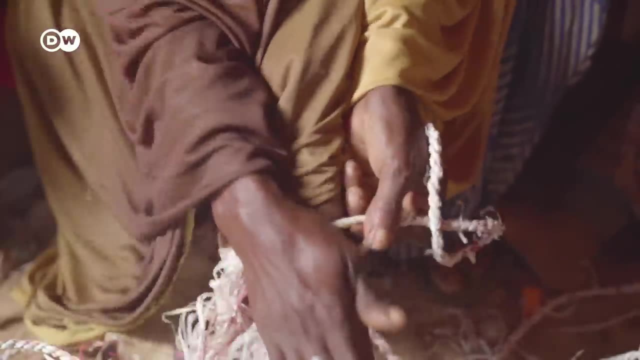 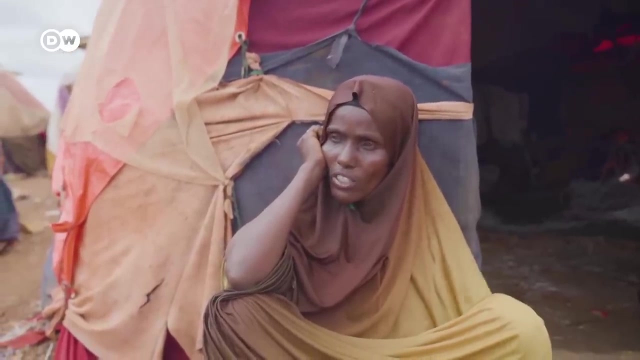 It's very hard living here. She tells us that a few weeks before Hawo Isaka fell ill, He had whooping, cough vomiting and diarrhea. The pills he was given didn't help any. He died because of the drought. We buried him 15 days ago. 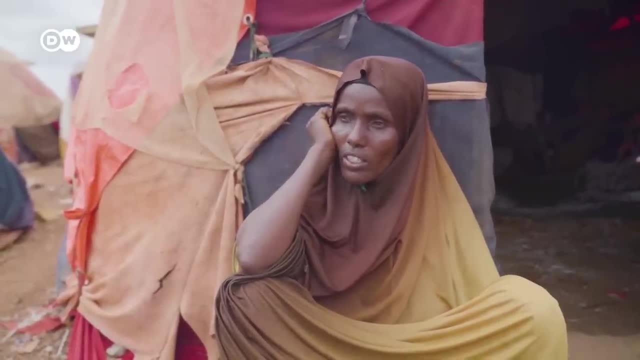 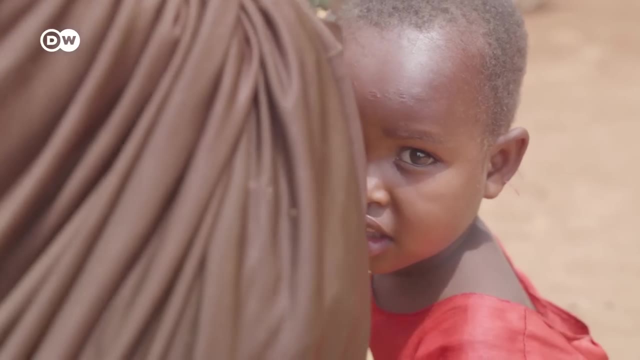 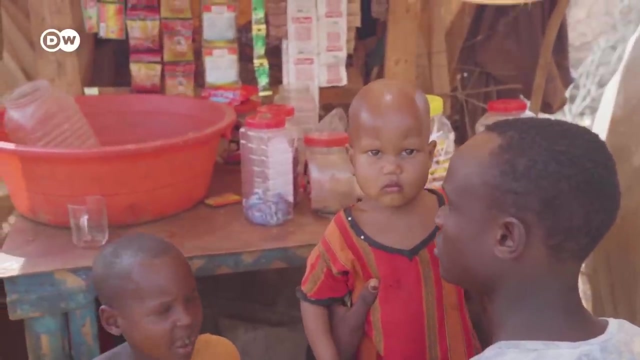 He was eight years old. The starvation got worse and so he died. The UN Children's Relief Agency, UNICEF, estimates that almost twice as many children will have died of hunger or starvation, But so far there are no dependable figures. We have half a million children. 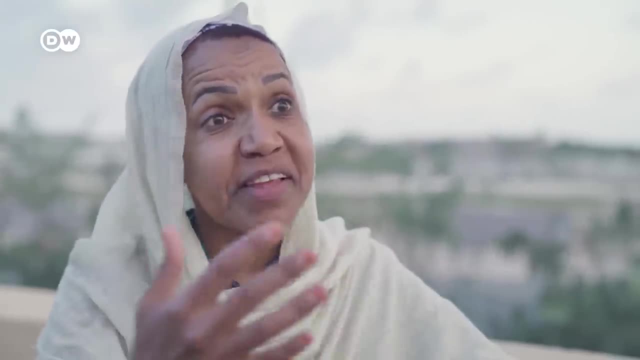 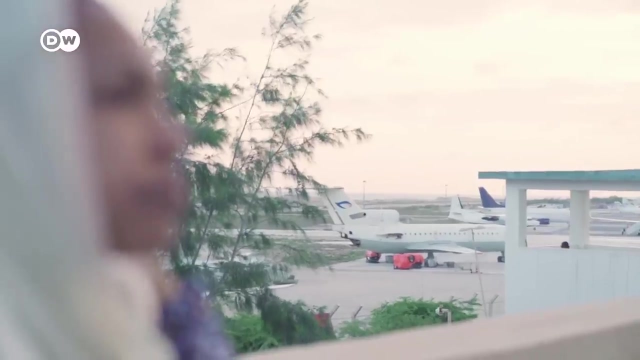 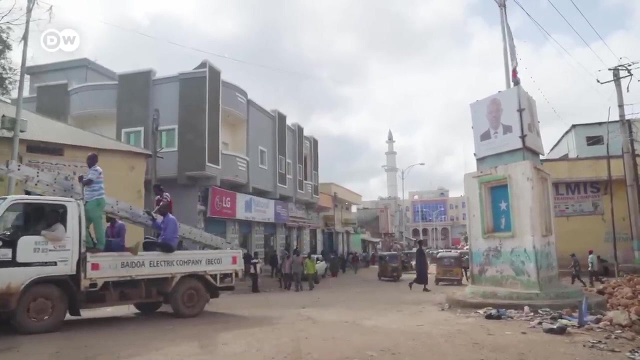 that are severely, acutely malnourished, which basically means that if they don't receive assistance timely, they are just simply going to die. According to the UN, one billion US dollars worth of humanitarian aid is urgently needed. Far more funding would be flowing. 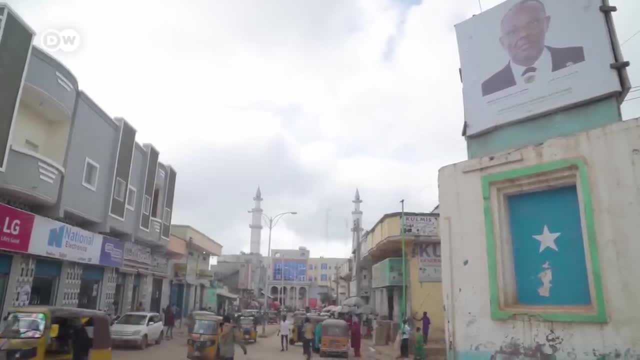 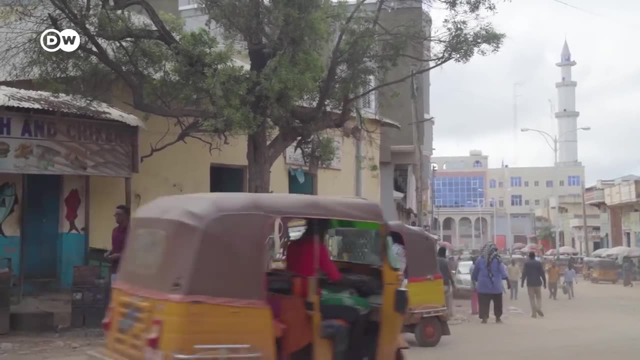 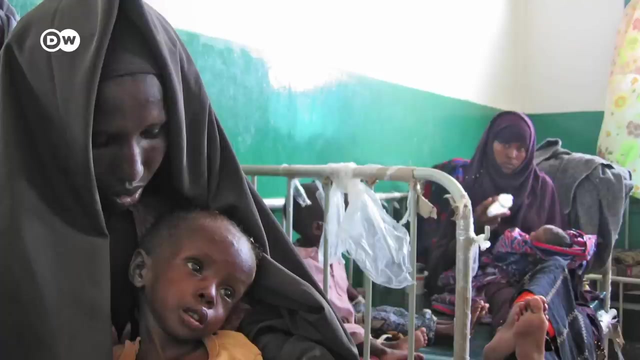 into the country if the Somali government officially declared a famine. The UN has agreed that such a move could enhance al-Shabaab's influence. Humanitarian organizations are warning that some regions have already crossed the threshold into famine conditions In 2011,. 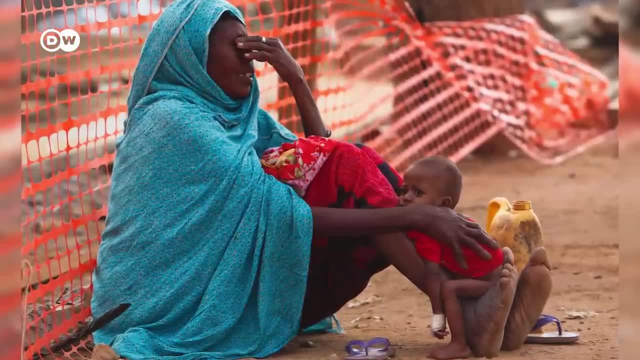 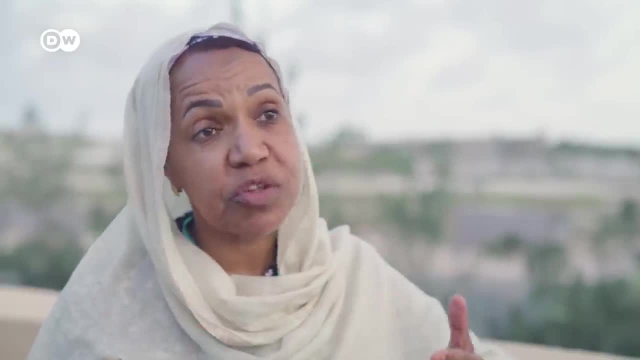 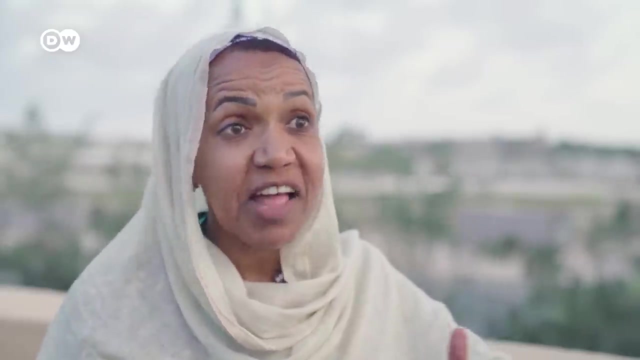 during one of the worst droughts in Somalia's history. over a quarter million people died, half of them before the famine was officially declared. We don't have to wait until 2011.. By the time famine was projected, already 260,000 people have died. 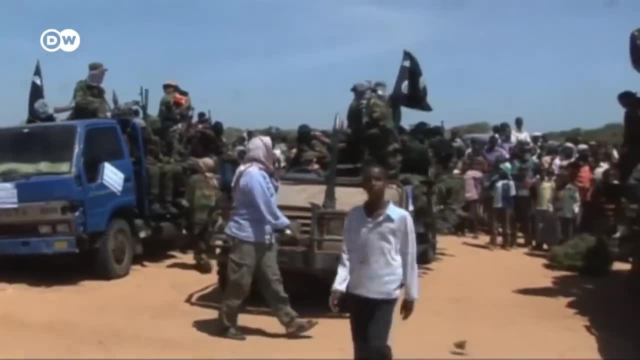 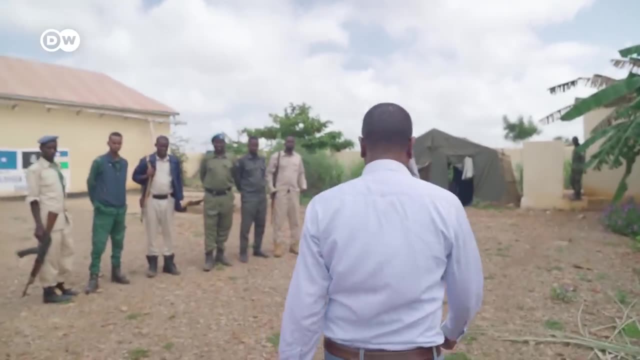 half of them are children. In 2011,, al-Shabaab held large parts of Somalia, making them inaccessible to aid. That included the city of Baidoa, This time Mayor Abdullahi Ouattine and Police Chief Mohamed Moukdar. 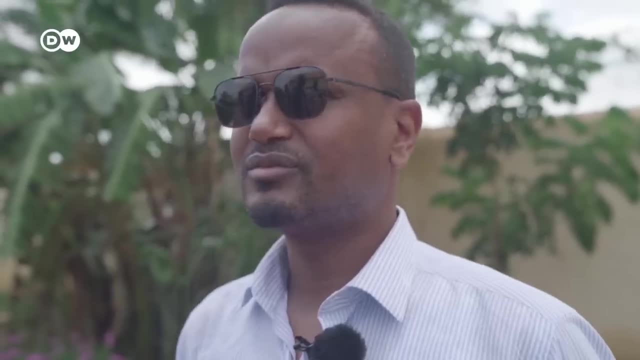 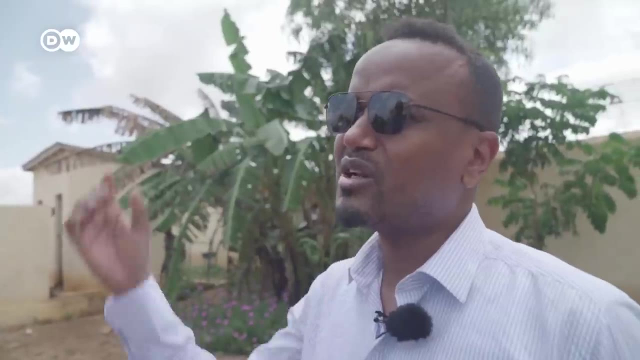 are doing what they can to keep al-Shabaab out. Even so, the militia isn't far away. We're at high alert, so we don't get ambushed. Have they let up at all? The pressure is let up somewhat. 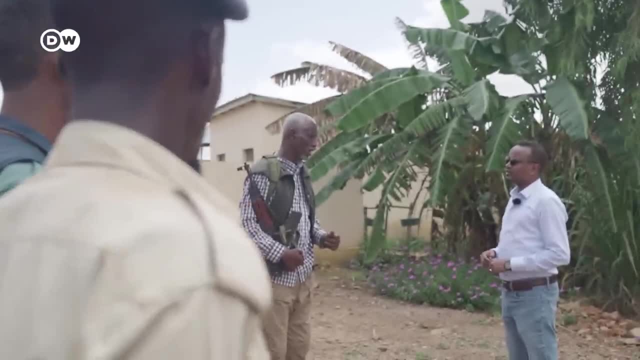 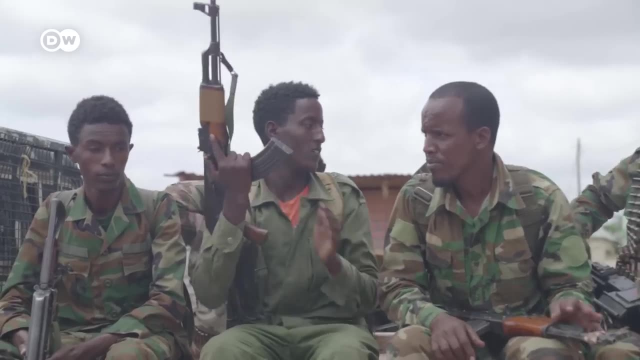 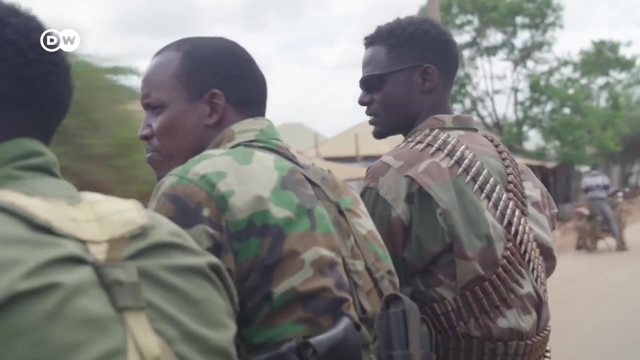 but yesterday evening it was bad. The al-Shabaab militias are present just 30 kilometers outside of town. Daily police patrols are designed to give people a feeling of security. al-Shabaab was the authority here until the government took the city back. 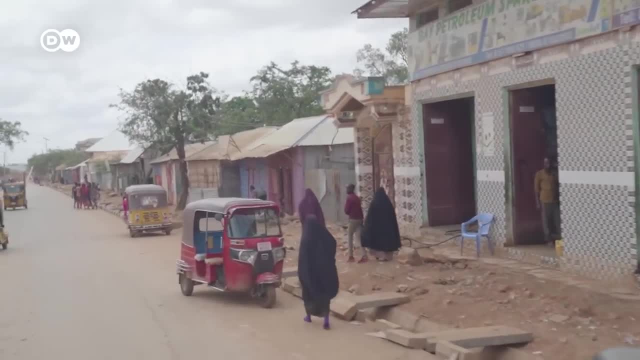 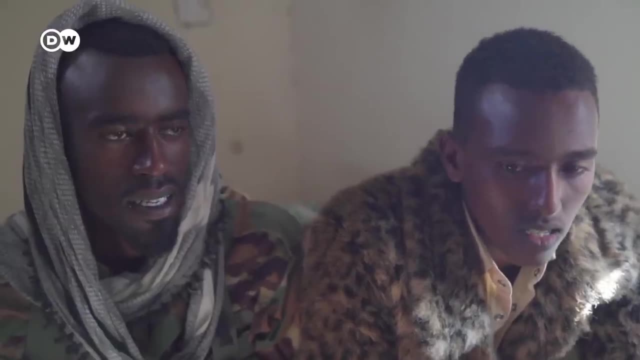 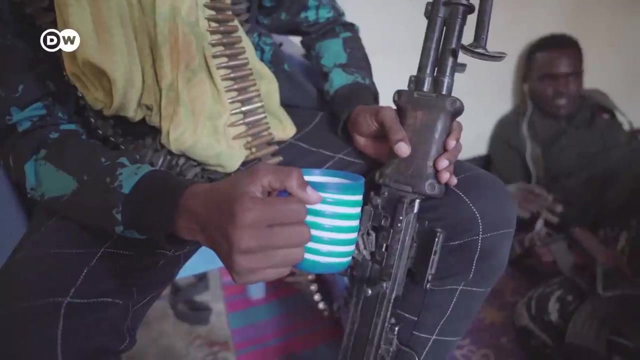 in 2012.. Militias loyal to the government like this one pitch in to help, And the population supports them. We met up with them in a hideout somewhere in Baidoa. Here they say they're planning their next attack on al-Shabaab. 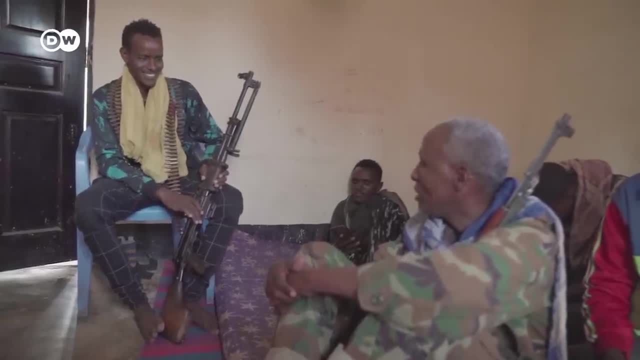 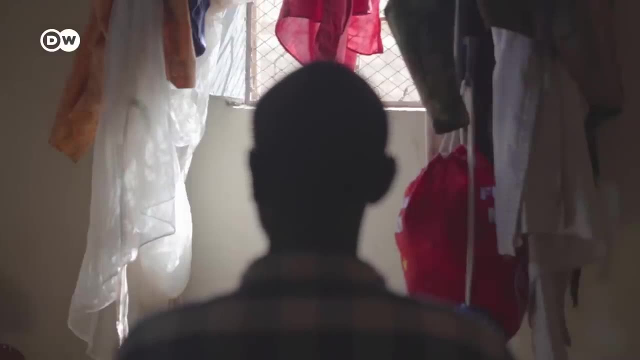 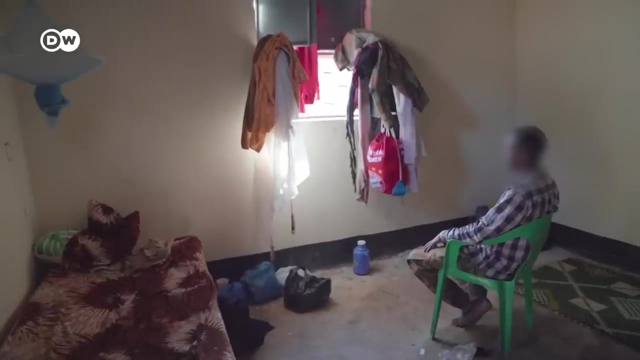 Their commander is a former al-Shabaab fighter himself. Back then, in my younger days, they had control of the country. There was a lot of unemployment and little opportunity. After a few years as an active fighter, he worked as a so-called tax collector. 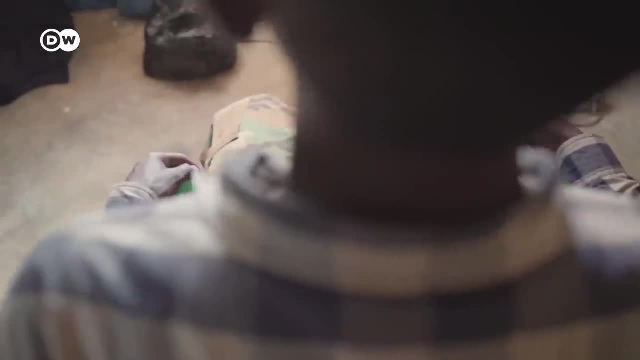 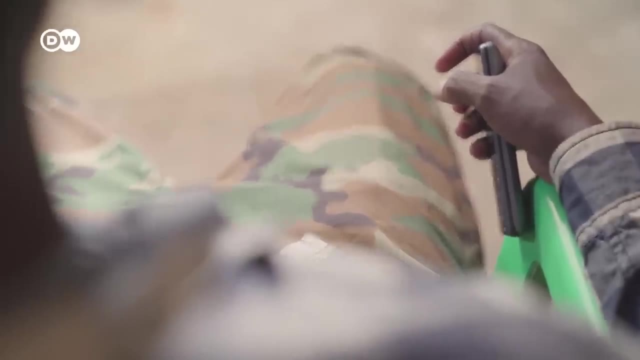 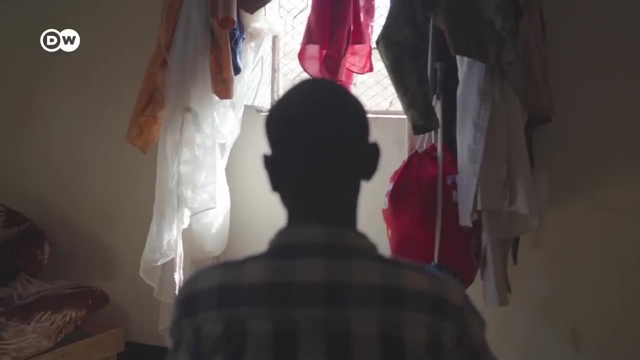 extorting money from shopkeepers and farmers, he says. But after almost 10 years in the group and witnessing torture and public executions, doubts begin to take hold of him. I realized they had no intention of establishing any government or rule of law. 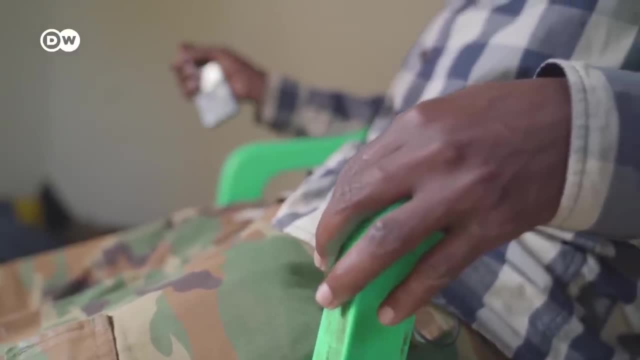 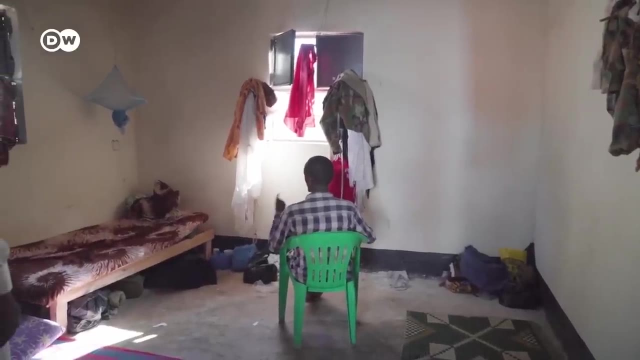 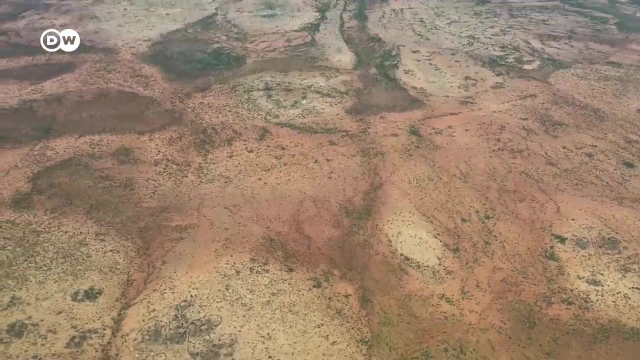 He had to leave his family behind. His wife was then forced to marry another fighter, And now he's afraid al-Shabaab will soon be recruiting his son into its ranks. They had no way to flee. Neither do about one million other people trapped in the areas. 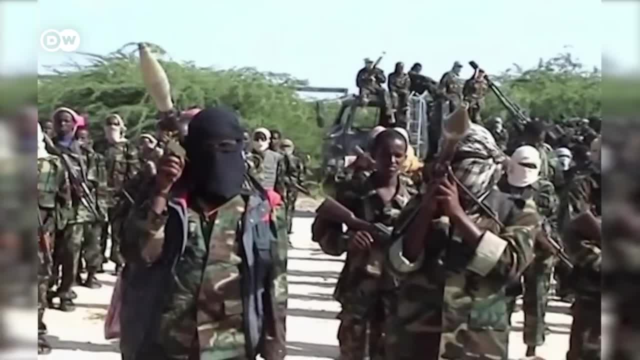 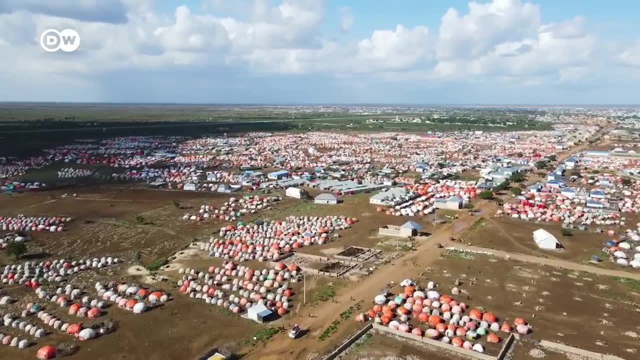 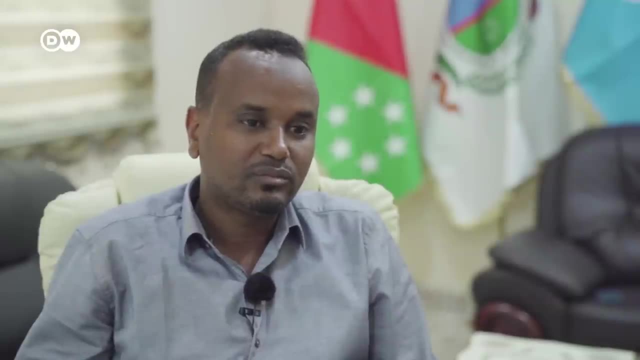 controlled by al-Shabaab, without access to aid. Al-Shabaab is aggravating the crisis, taking what little the starving population has left and holding them hostage in their territories. Aid organizations are warning that most of the famine's victims could be in these areas. 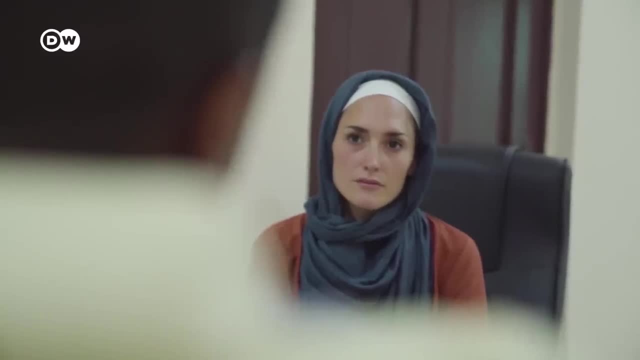 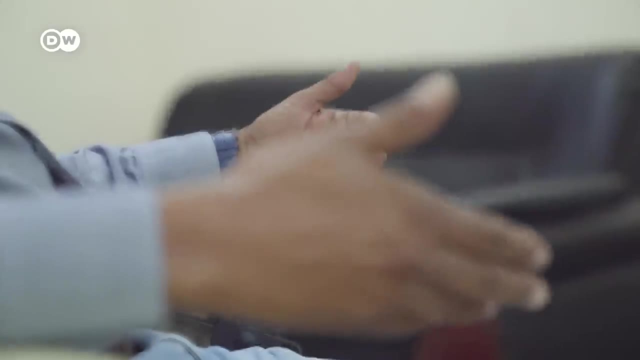 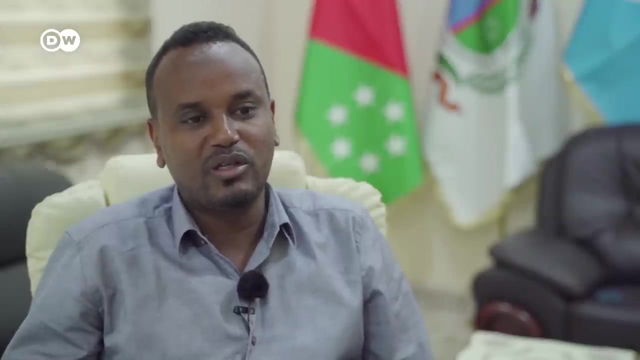 Baidoa's mayor Watin says he's had enough short-sighted solutions. Somalia is one of the affected areas by the climate change, But what will happen after the drought ends? Do we wait until another famine comes, Or do we still come up? 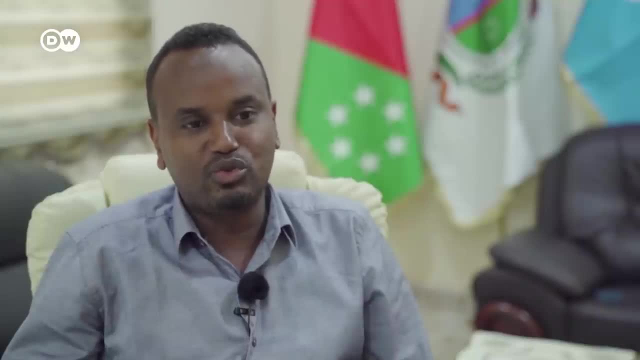 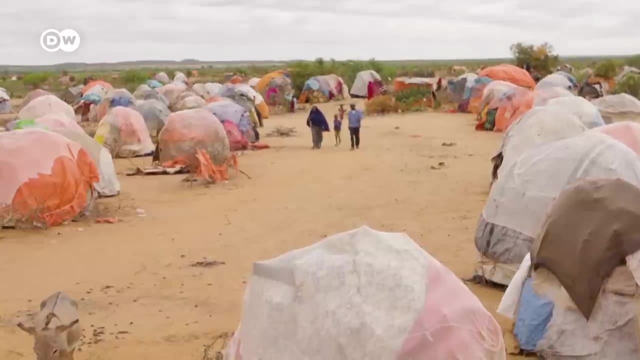 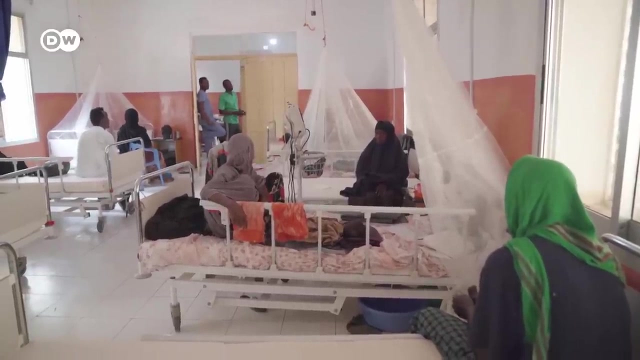 with initiatives that will mitigate future shocks. African countries together contribute less than 3% of all global greenhouse gas emissions, Yet they are the worst affected by climate change, And the first to feel those effects are the children In Baidoa's hospital.